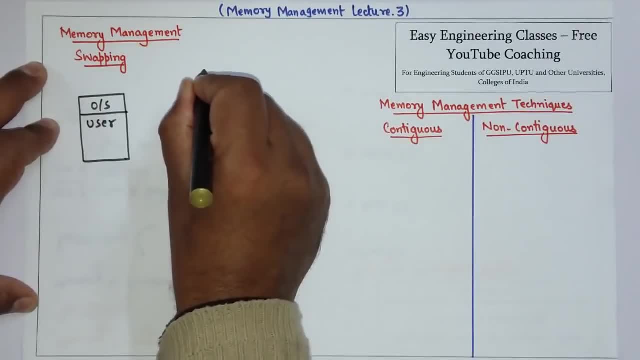 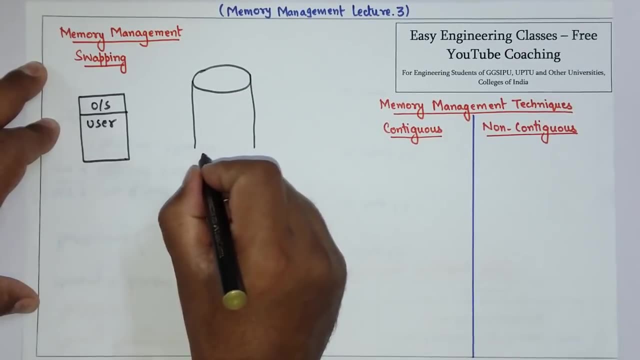 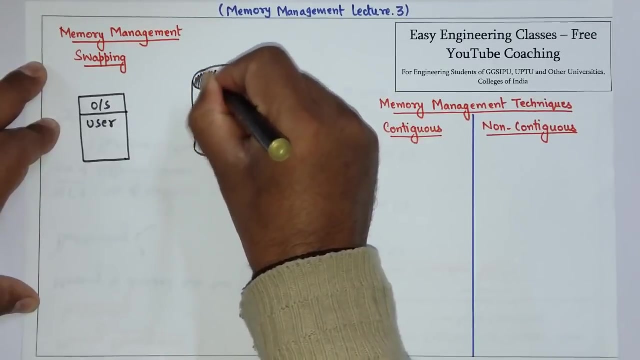 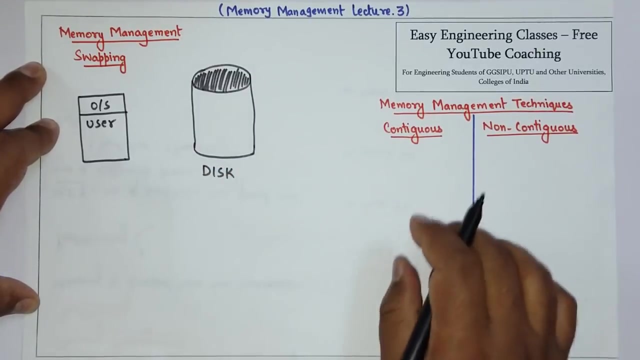 n number of processes. We have many processes in the disk and we have to run all those processes in main memory. So the space is limited. Suppose this is the main memory, this is the disk and in this disk there are many processes, or you can say there are jobs. 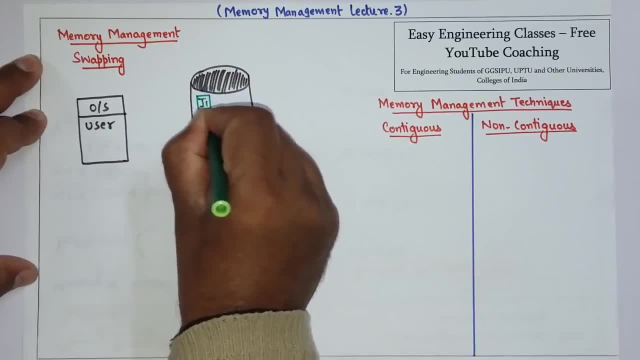 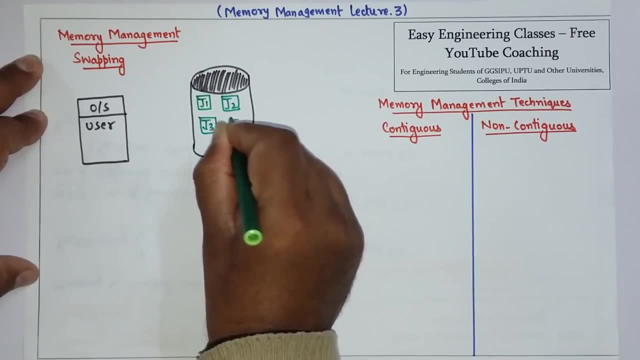 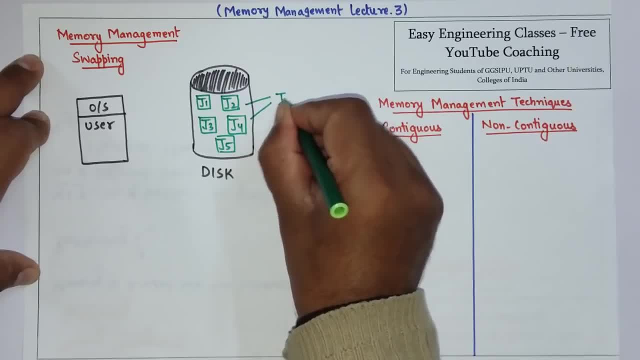 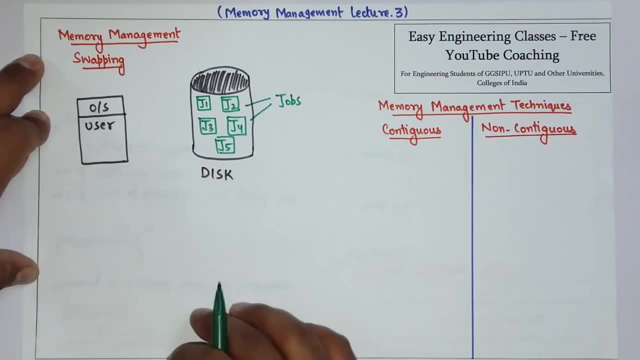 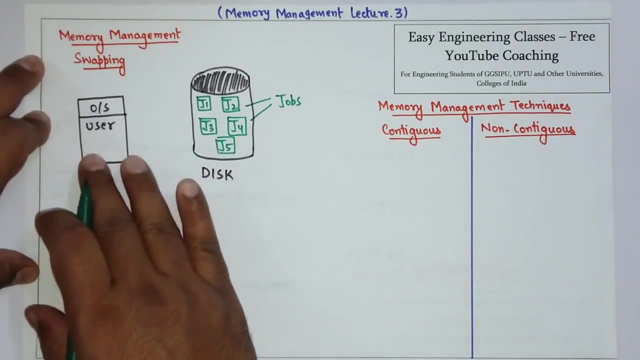 J55.. So we have 5 jobs here that are waiting to be executed in the physical memory. Now the space of the physical memory is not enough to execute these 5 jobs or 5 processes together. So what happens is that the jobs come in one by one and are executed. 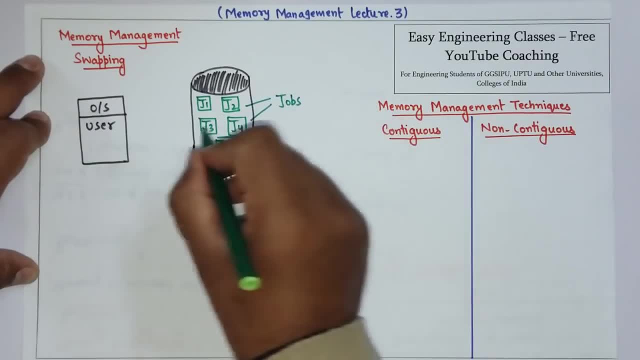 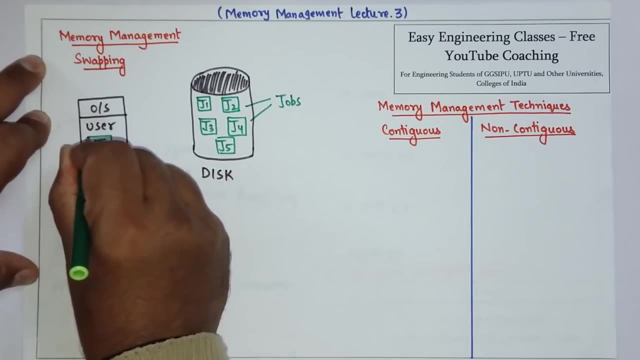 Suppose we have a physical memory. So the first job that we got to execute was J1. So what we have done is we have allocated the area here to J1. Now J1 is being executed here in the physical memory space. This is the physical memory. 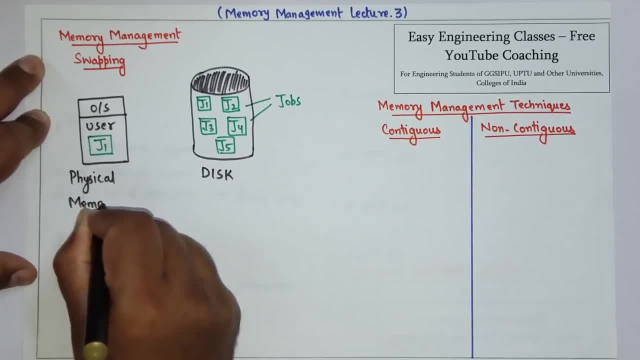 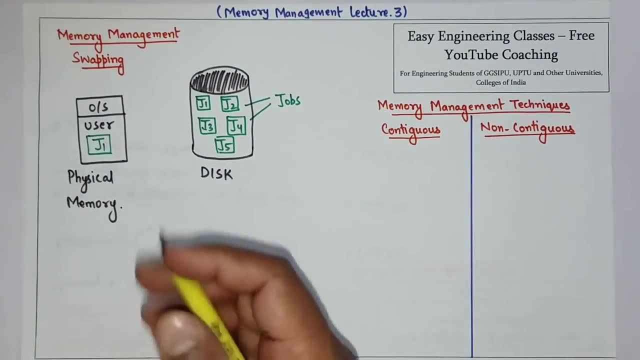 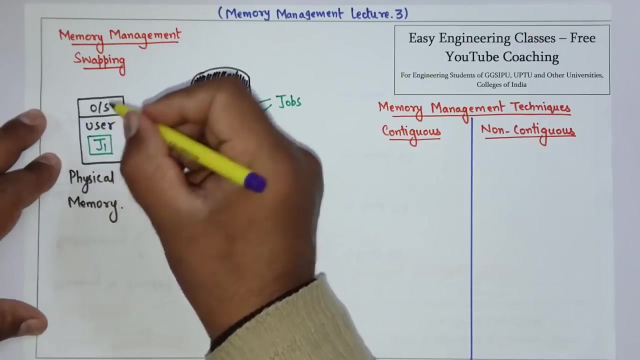 So J1 is being executed here, and when the execution of J1 is over, then we will remove it from here. Now, where will we send it back? In the disk? So the process that takes the job from physical memory to disk after completion of its execution. 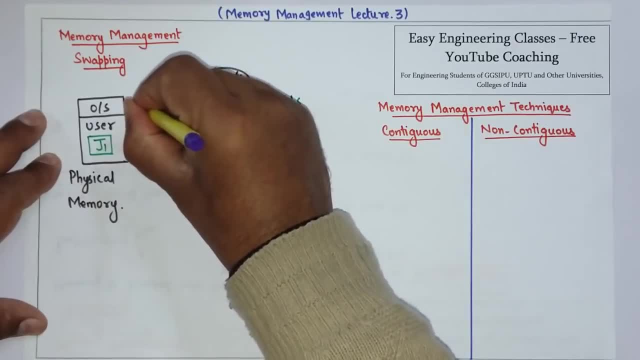 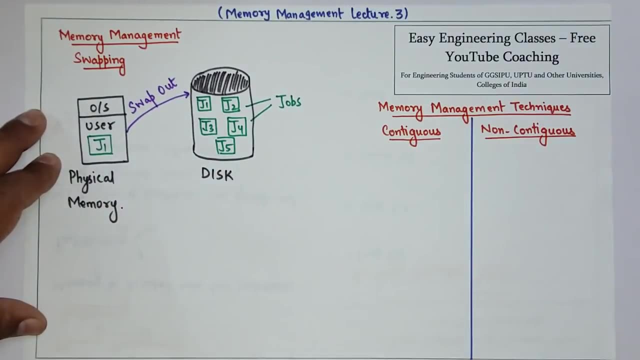 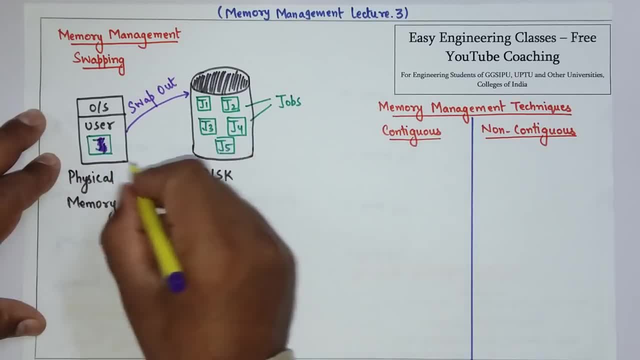 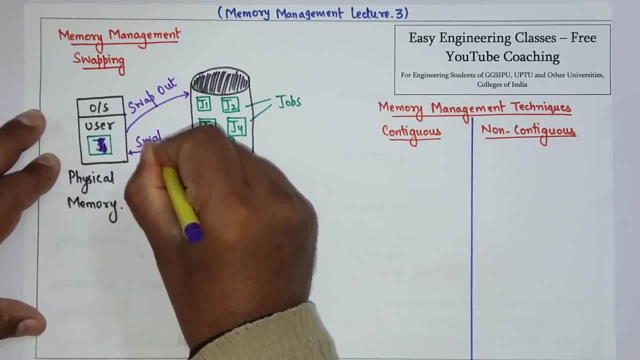 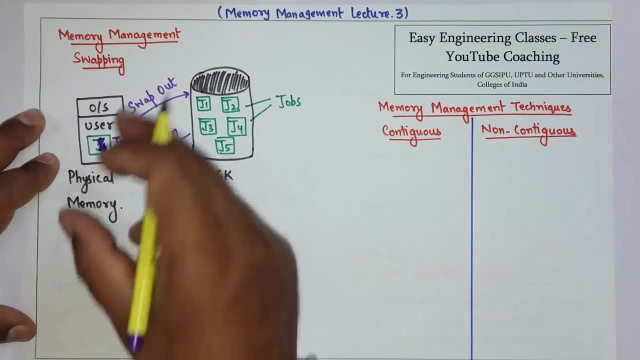 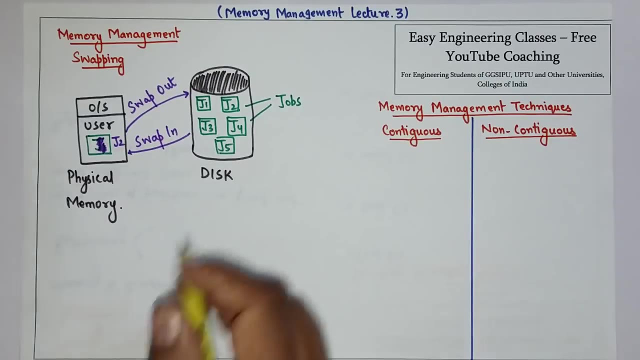 So what we have done is we have SwapIn J2.. We have Swapped In J2 in the main physical memory And the process of this SwapOut and SwapIn is known as Swapping. So this is Swapping In. this you can write when J1 is entered: 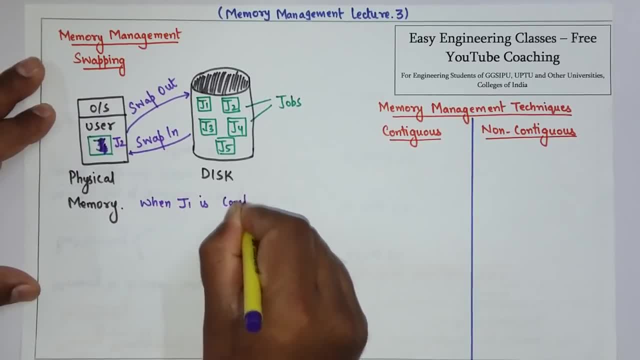 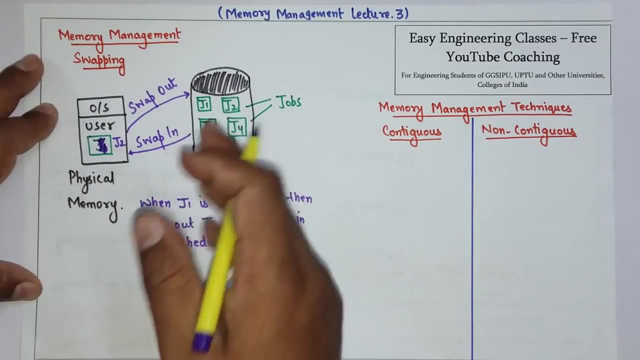 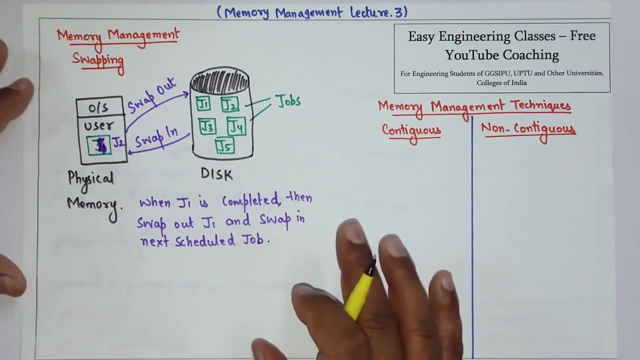 Then j1 is completed, then swap out, then swap out j1 and swap in next scheduled job. So swapping is a process of swapping out and swapping in of processes or jobs from the disk to the physical membrane and vice versa. So this is the basic idea of swapping. 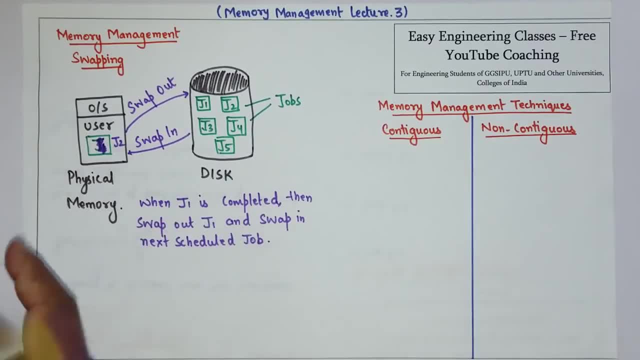 Now there is one more variation of swapping, which is sometimes known as roll out, roll in process. So now we will going to discuss about that. So the variation that we are talking about swapping is known as roll out, roll in. So the variation that we are talking about swapping is known as roll out, roll in. 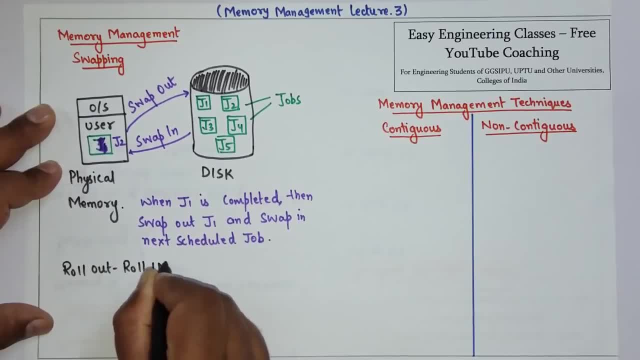 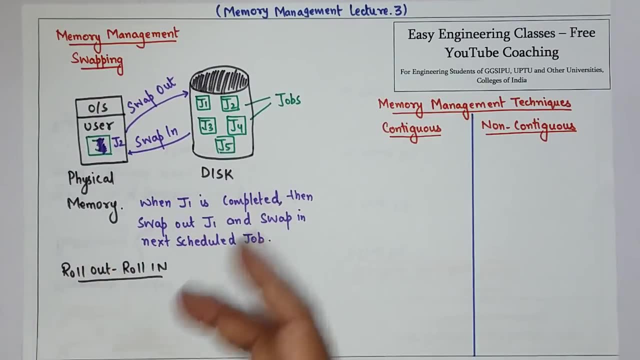 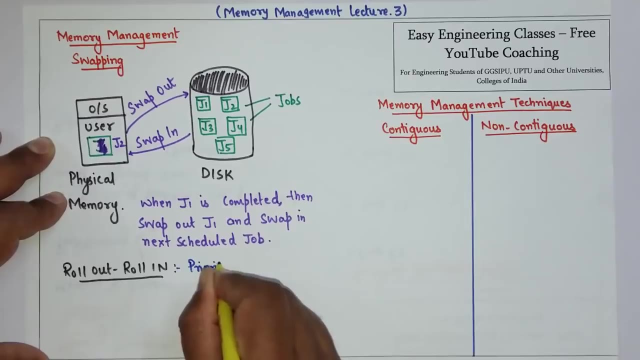 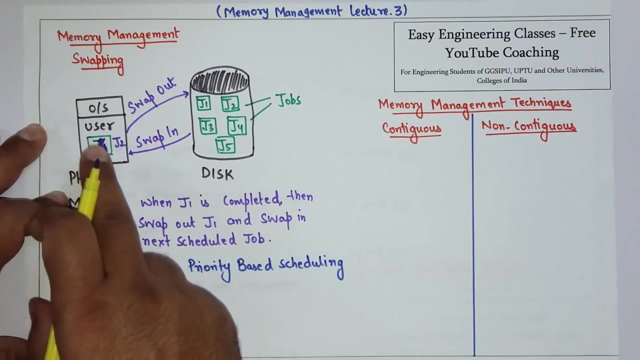 And in this roll out, roll in, what is done is: it is based or it is used for priority based scheduling algorithms. So it is basically a priority based scheduling algorithm. Now let's see what we were doing. So when a process or a job's execution was getting over, then we were swapping it out. 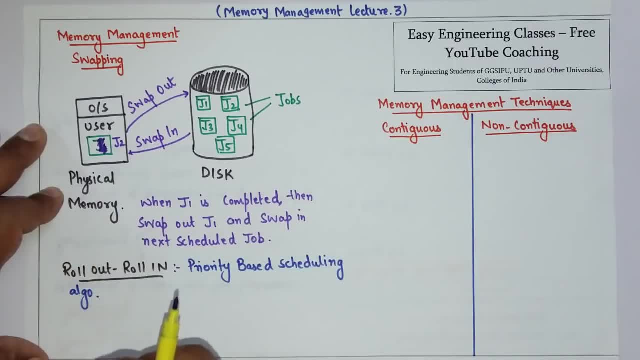 Now in the variation of swapping, that is, roll out and roll in if a higher priority process arrives. So if a higher priority process arrives and wants service of the memory, then the memory manager can swap out a lower priority process and execute the higher priority process. 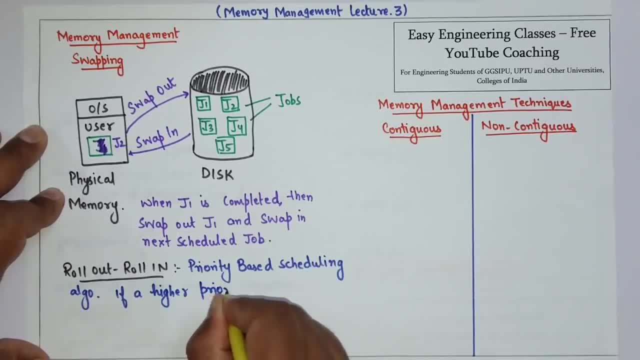 So if a higher priority process, for example J4, arrives, then a lower priority process, then a lower priority process, for example J2, will be roll out and memory manager can switch out. So if a lower priority process, So if we look at that, 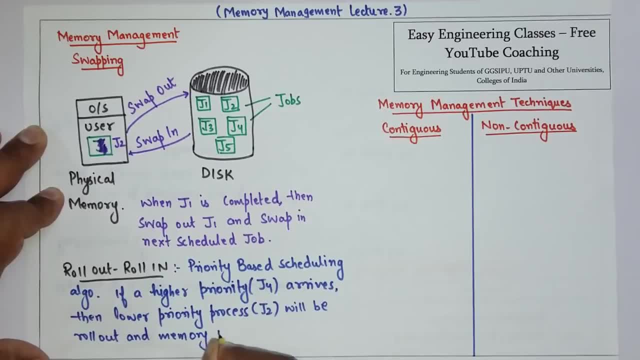 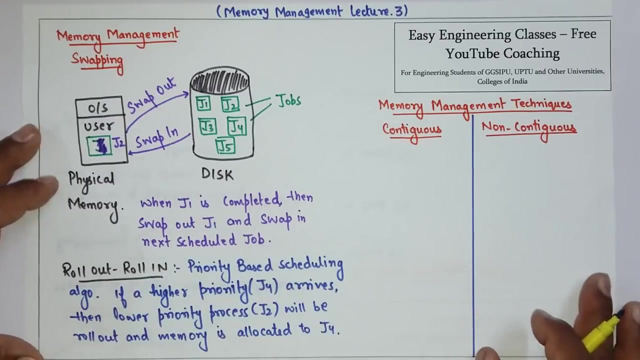 memory is allocated to the higher priority process, So it has not wait for the completion of J2.. So that is a variant where the completion of job is not taken into account, but the priority of the job is taken into account and the processes or the jobs are roll out and roll in based 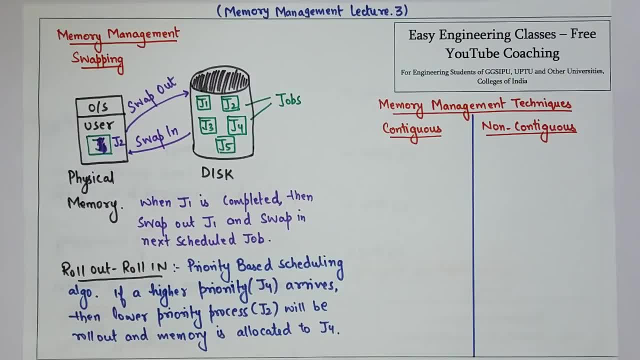 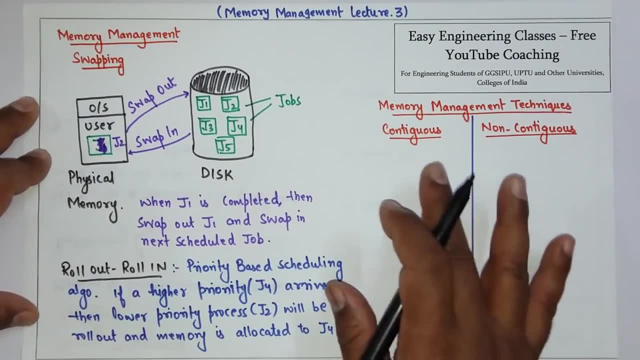 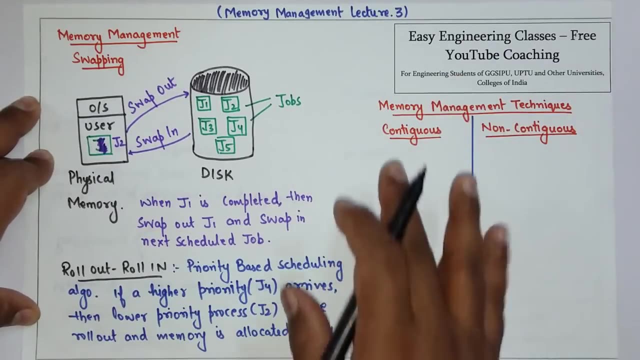 on the priority. So this is about the swapping and next we will see about the memory management techniques. So basically there are two different types of memory management techniques. One is contiguous and another is non contiguous- Detail we will discuss in next lectures. In this lecture I am just writing about the difference between them. 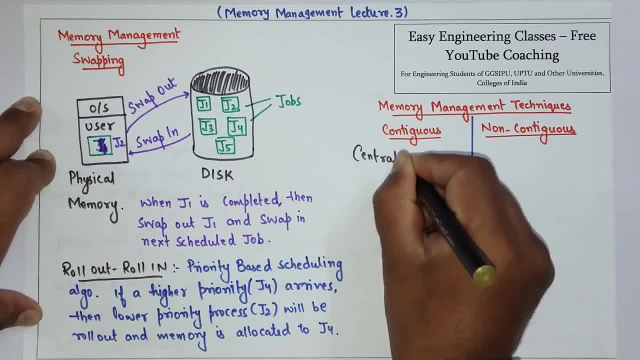 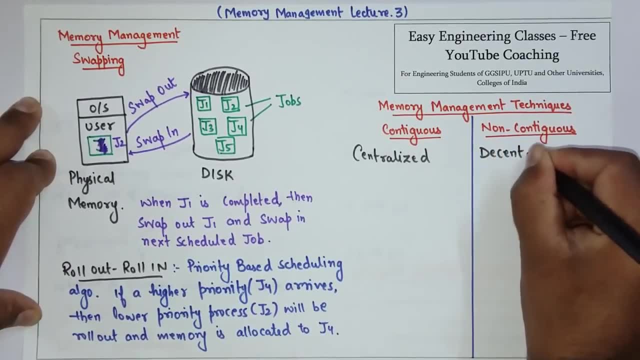 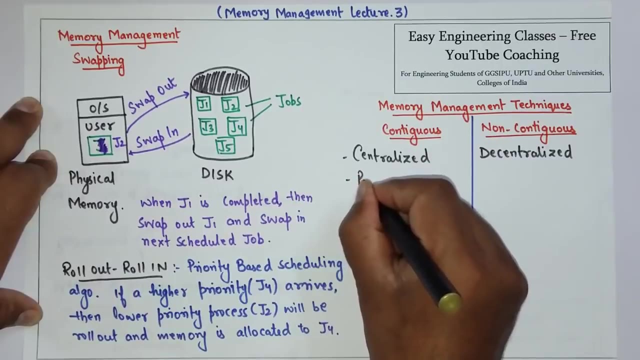 So the contiguous is centralized in nature. It is centralized in nature, Whereas non contiguous is decentralized. So this is about the swapping. Next we will see about the memory management techniques In this a program. in this a program or process as a unit is, as a unit is completely stored. 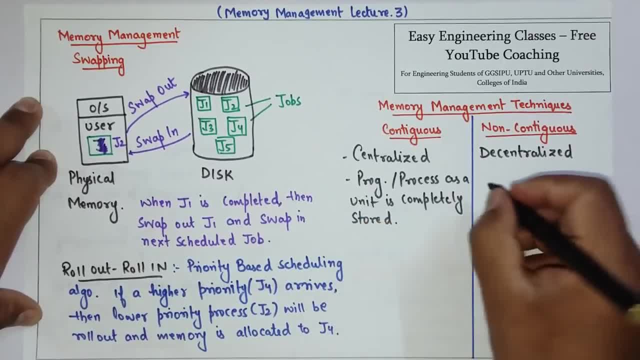 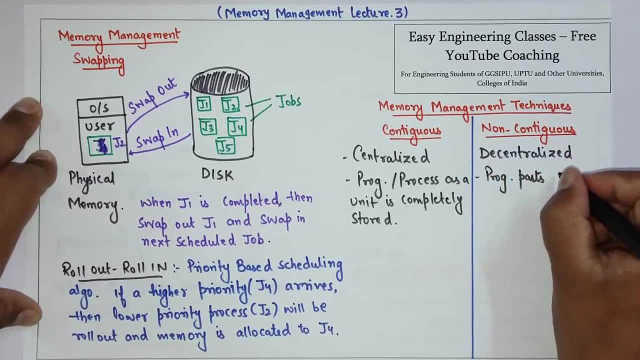 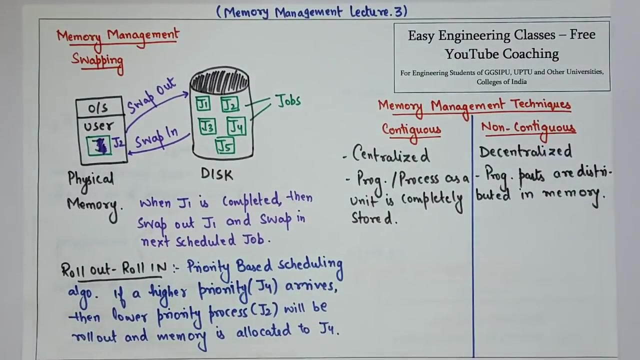 in this a program or process as a unit is completely stored, whereas in this program portions or parts. In this program, portion of parts, Are distributed, Are distributed, Are distributed in memory. In this program or process it is stored as a whole unit, whereas in non contiguous, the parts. 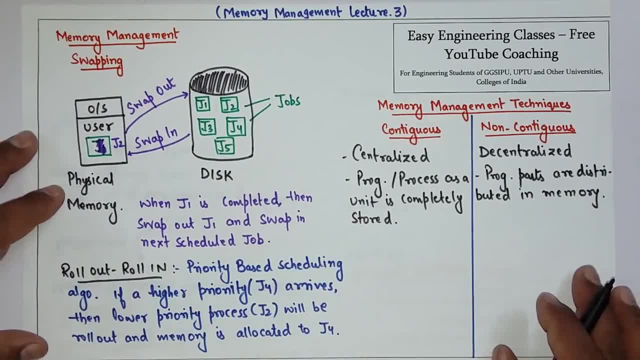 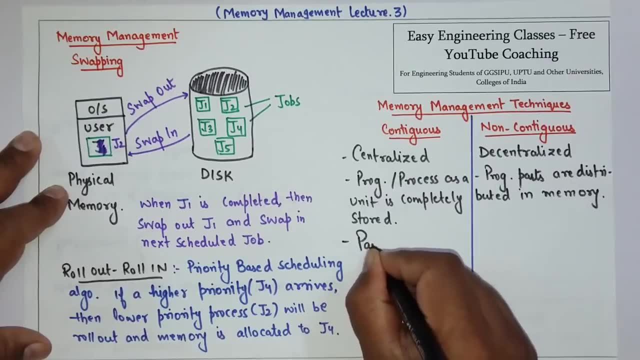 of the program are distributed in memory And contiguous are contiguous. memory management is implemented with the help of partitioning method. Contiguous are all the parts. Contiguous are all the parts. We will see in detail about the partitioning in the memory management, lecture 4..